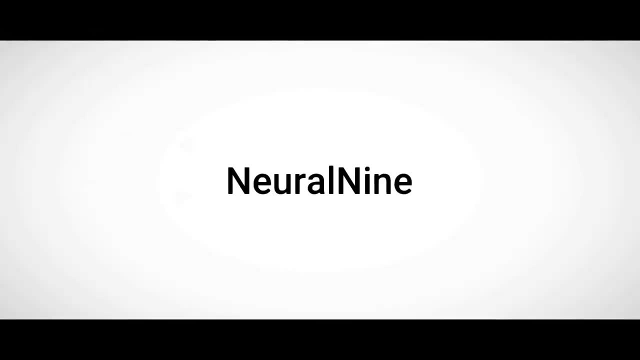 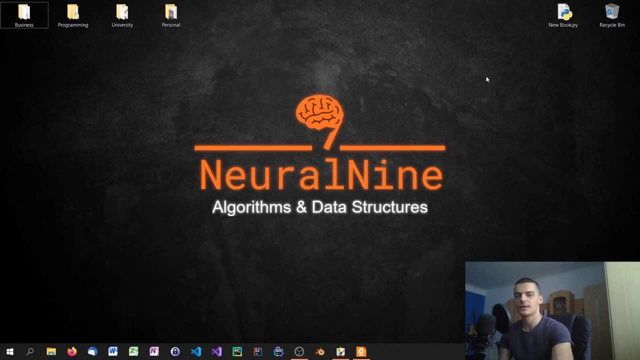 What is going on, guys? welcome back to the algorithms and data structures tutorial series, and today we're going to talk about the Kruskal algorithm, which is the algorithm for finding maximum and minimum spanning trees in graphs. So let us get right into it. So let's start looking. 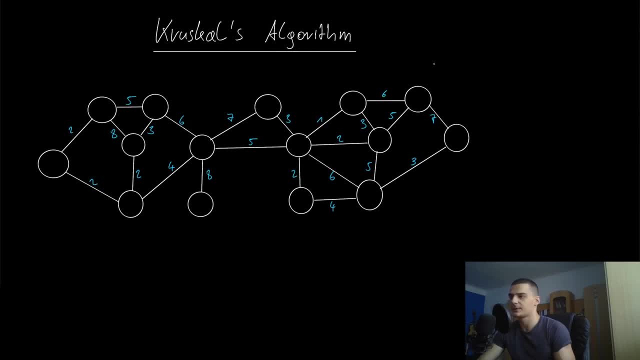 at this graph here and don't be confused. yes, it's a little bit larger than the graphs that we looked at before, but it's, yeah, the Kruskal algorithm. it's very simple. so we need a large graph to show what it does, and it's again a weighted graph here, so it has to be weighted, of course, because we're 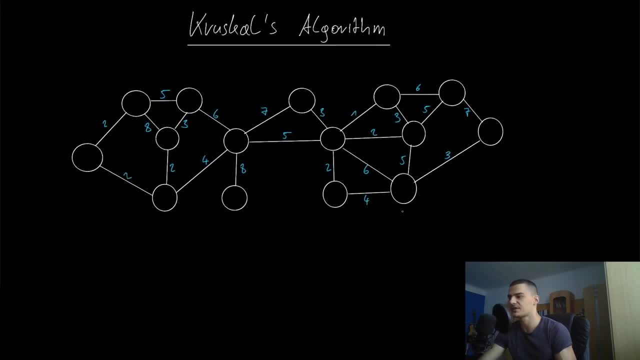 looking at a minimum or a maximum spanning tree, and a spanning tree is essentially just choosing all the edges that cover all nodes. so essentially you want to end up with a bunch of edges that cover all nodes so that all nodes are interconnected and we can get to every node. 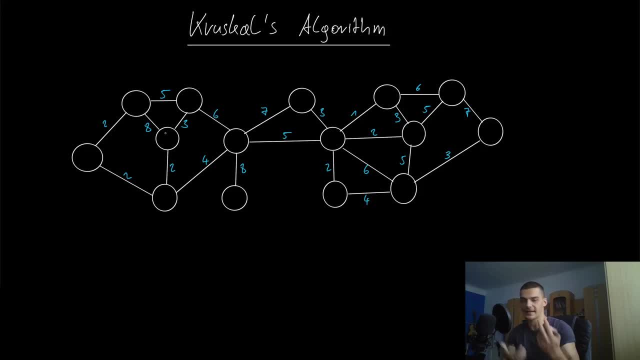 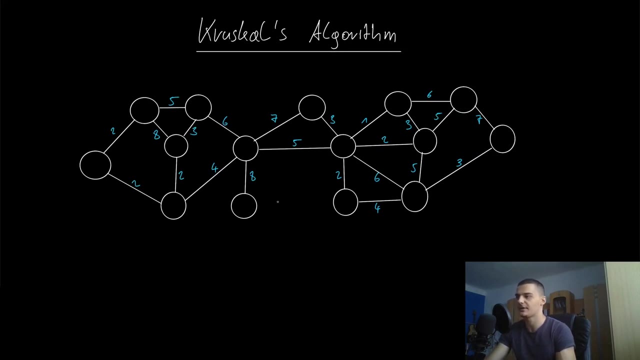 with a minimum amount of cost or a maximum amount of benefit whatever, in whatever way you interpret these numbers. so if this is, if these numbers represent the amount of money you get when you go there, you want to maximize it. if they represent the distance or the amount of money you have to spend to get there, the cost you want to minimize. 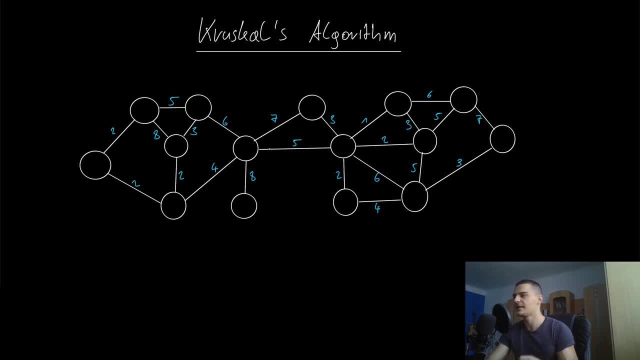 them. so we want to end up with a tree where we can remove all the edges that we don't care about, all the edges that are inefficient, and we want to end up with a minimum spanning tree. so to say now, for example, what we could do without applying the Kruskal algorithm, we can just go ahead, for example, and delete this. 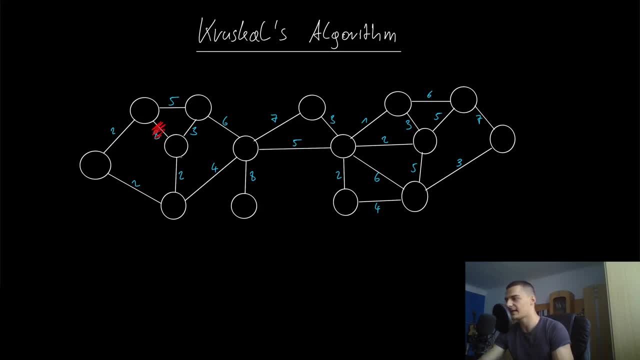 edge here because obviously we don't lose any nodes because of that and it's a very high cost edge, so to say. we cannot remove this edge here, even it has, even though it has a cost of eight, because there's no other connection to this node. so we get the idea of what we're looking at and 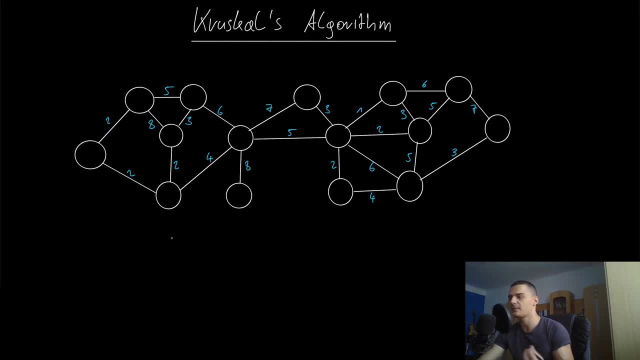 the Kruskal algorithm is actually very simple. if we're looking for a minimum spanning tree, we're just looking at the minimum cost edges and choosing those edges as long as they don't build any circles. so, for example, if I were to choose the one here and to choose the two here, I could not choose the three anymore because it would close. 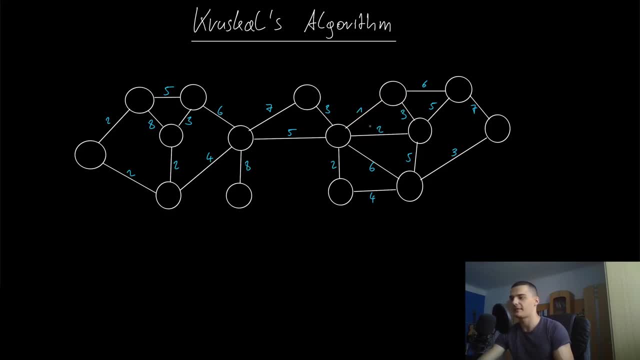 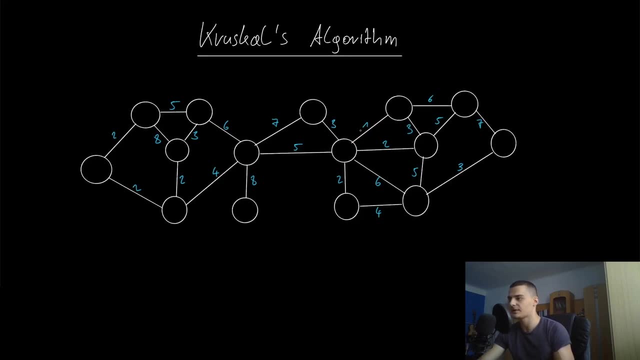 a circle, it would go ahead and close a circle, and we don't want to have any cycles, circles or whatever in here. so what we need to do here is we just start with the smallest values, so one, for example, or not for example, one in this case- and we choose this edge. so we have one edge already: that 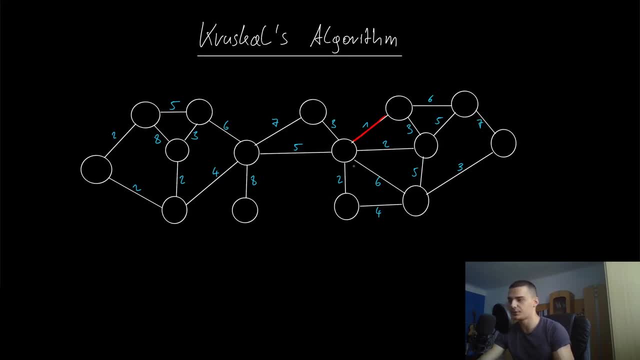 and we don't find any other ones here. so we proceed with twos and we mark all the twos. so this is a two, we select this edge. let me just make this a little bit thicker here. maybe I can use a line tool like that. yes, so we choose this one. we choose this one first, of course. then we also choose this: 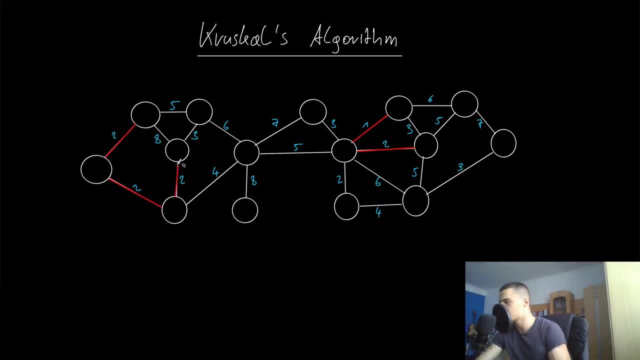 one and this one, and this one and, of course, this one. all the twos are just being chosen and then we have no twos left, so we proceed with the three. we choose this three here. we choose this three here. as we already said, we're not going to choose this three here because it closes a circle. 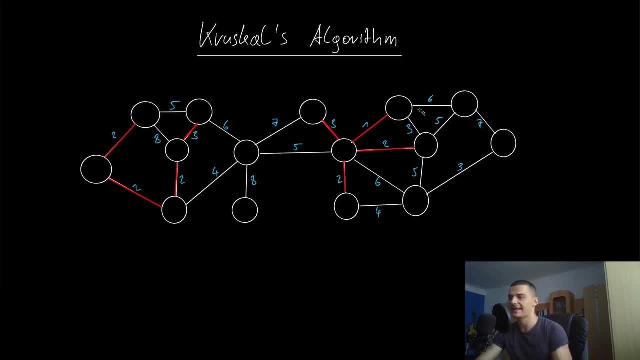 we're not interested in that because- think about it- we're not getting any benefit. we already have this node covered, this node covered, this node covered. sorry, adding this edge doesn't give us any benefits. it just connects these two nodes, but they're already in our spanning tree, so we don't. 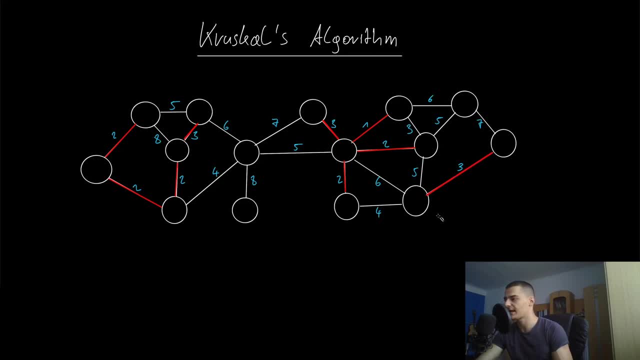 care about them. then we choose this edge and the threes are done. we proceed with the four. we choose the four here, it doesn't close a circle. we choose the four here. it doesn't close a circle, and that's essentially it. then we go to five. we don't choose this five here because it closes a circle. if we choose this, 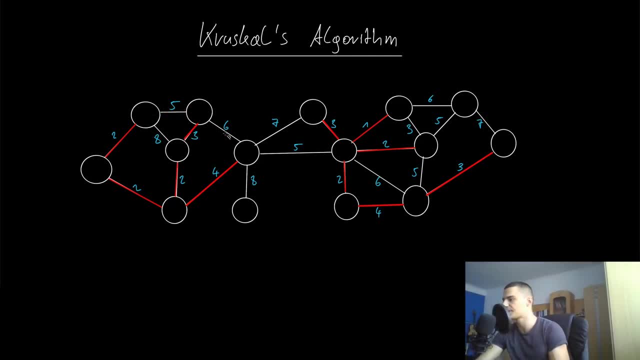 five here. you can see that this circle here is closed, so we don't choose it. we choose this five, however, because it does not close a circle and it's important to connect these two graphs. this would close a circle. this would not close a circle, so we use it. we choose it, then we proceed with the. 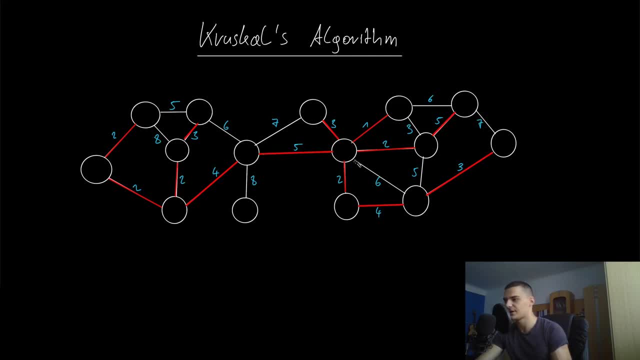 six. we don't choose this six because it closes the circle. we don't choose this six because it closes the circle. and we don't choose this six because it also closes the circle. so we don't choose any six. here we have seven. this seven here closes a circle. this seven year closes the circle, so we don't. 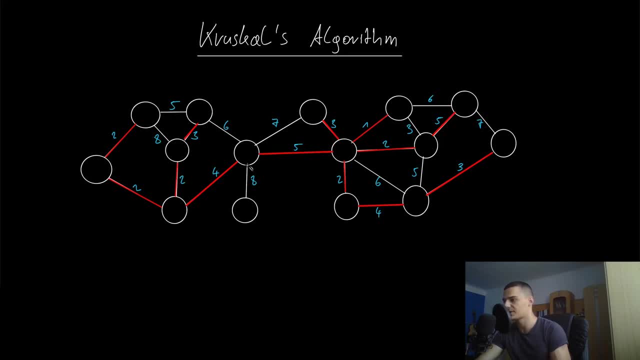 choose this six because it doesn't close a circle. we only left with the eight. this eight closed the circle and, as i already mentioned, this eight here is mandatory. even if it was a thousand, we would have to choose it because there's no other way we can include this note and this is the result. 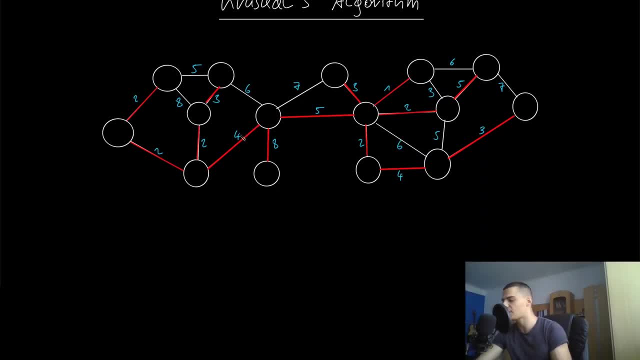 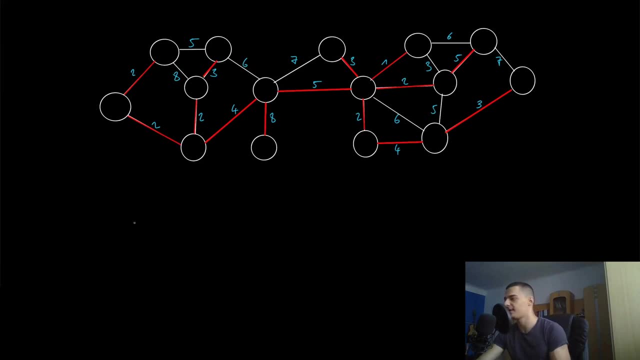 essentially, if i didn't miss anything, every node should be covered and we could now go ahead. i'm not going to do it completely, but we can now go ahead and, uh, rewrite or redraw this graph here by having all the notes that we just had, all the same notes. 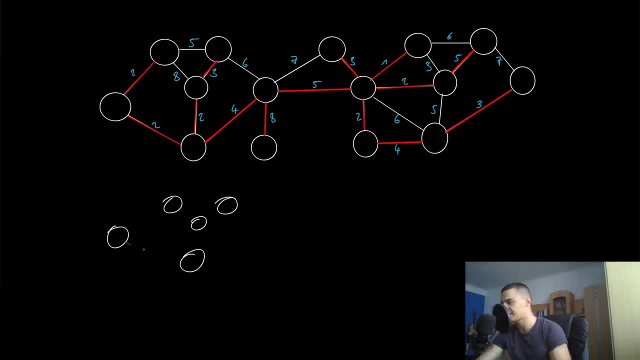 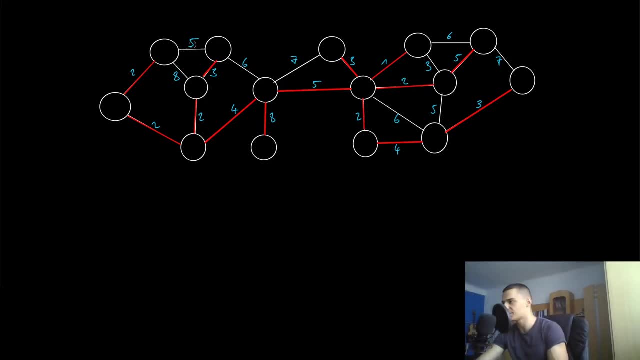 way would just be to delete the edges. so we could just go ahead and- uh, let me choose the delete tool here- could just go ahead and delete all these edges here and we would end up with the minimum spanning tree for this graph. so, all nodes that are not, all edges that are not selected. 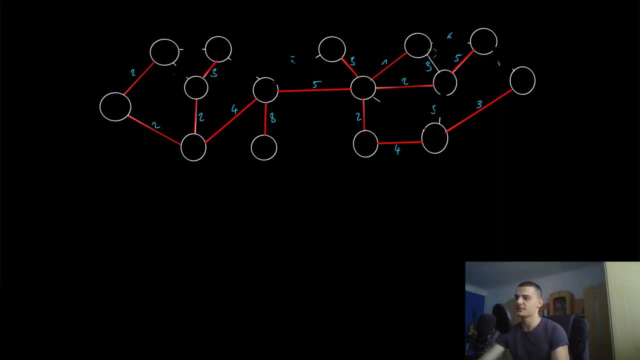 are deleted, and we would end up with this minimum spanning tree here, this one too, where all the nodes are connected, interconnected, with the minimum amount of cost. we can do the same thing for the maximum amount of cost. the only thing that we need to do, then, is we need to start with eight. 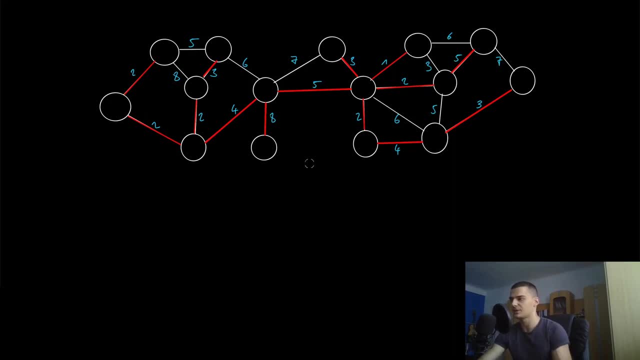 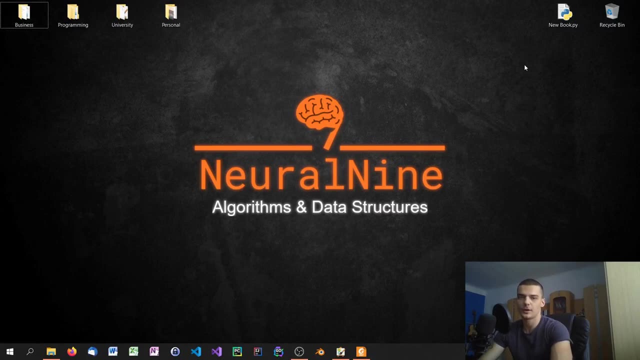 and go uh and decrease the value with each iteration, so to say. this is the basic cross calls algorithm algorithm. so that's it for today's video. i hope you enjoyed it. i hope you learned something. if so, let me know by hitting the like button and leaving a comment in the comment section down below. 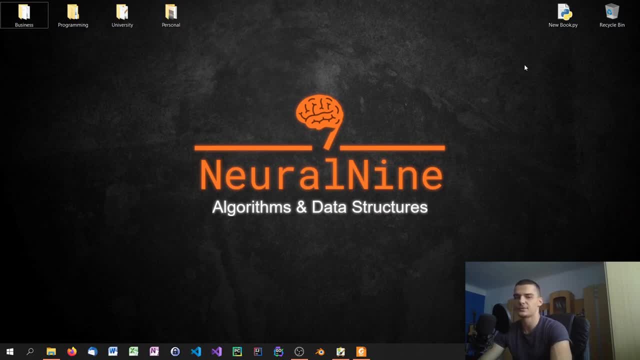 uh, we're now done with the graph theory. we're going to proceed with the data structures. in the next video we're going to start with linked lists, stacks, heaps and all these data structures. we're going to talk about them, analyze the runtime complexity, the runtime complexity of their 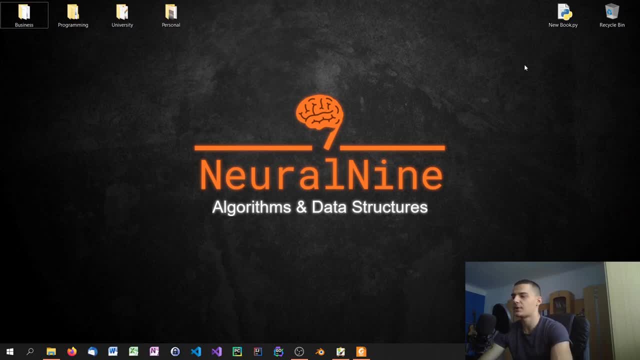 operations. uh, and we're now done with the graph theory. so, um, that's it now again. if you have any questions, if you want to leave any feedback, feel free to do so in the comment section down below. also, make sure you subscribe to this channel if you want to see more future videos for free. other than that, thank you very much for watching.